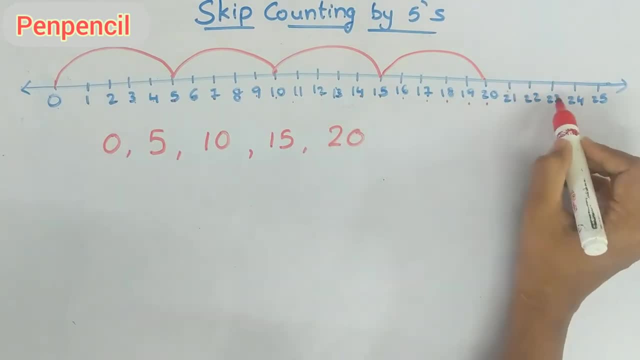 In this way, you have to do skip counting 1,, 2,, 3,, 4,, 5. 25.. Like this, you have to learn skip counting by 5s. Okay, Now we will do few worksheets so that we can learn them easily. Okay, kids. 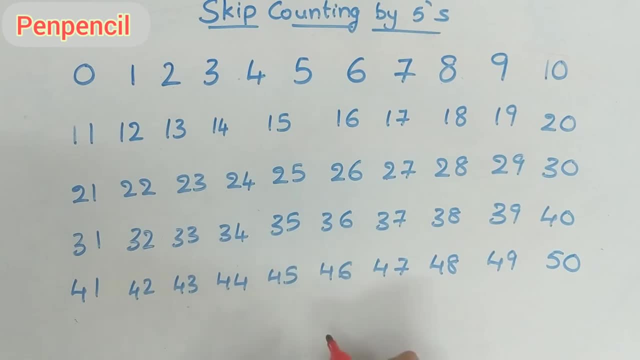 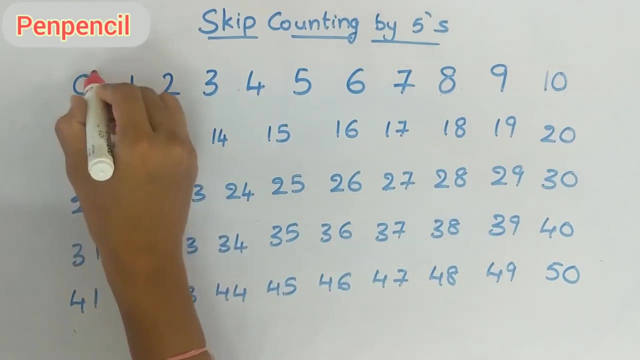 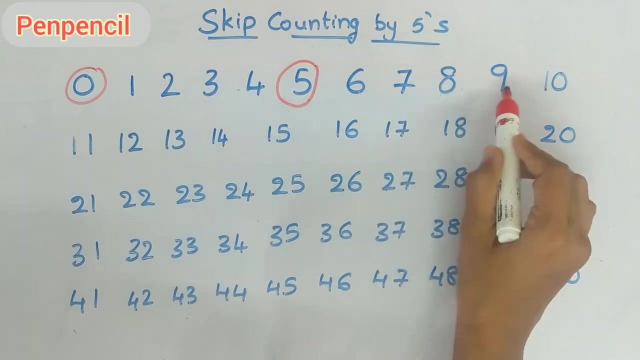 Okay, kids, Now you have to circle the numbers. Skip counting by 5s. You have to circle, Okay. Now come on, let us start. First number is 0. Next, 5.. Next you have to count it as how I have said: Okay, 5.. After 5,: 1,, 2,, 3,, 4, 5.. So after 5, the number is 10.. Now you have to count what is the number after 10 by skip counting by 5s: 1,, 2,, 3,, 4, 5.. 15 is the number. Very good. Now. next number is 10.. After 10, you have to do skip counting by 5s: 1,, 2,, 3,, 4, 5.. 15 is the number. Very good. Now. next number is 10.. After 10, you have to do skip counting by 5s: 1,, 2,, 3,, 4, 5.. 15 is the number Very good. Now. next number is 10.. After 10, you have to do skip counting by 5s: 1,, 2,, 3,, 4, 5.. 15 is the number Very good. Now. next number is 10.. After 10, you have to do skip counting by 5s: 1,, 2,, 3,, 4, 5. 15 is the. 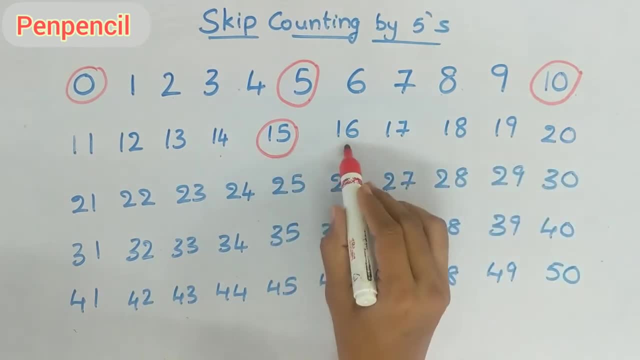 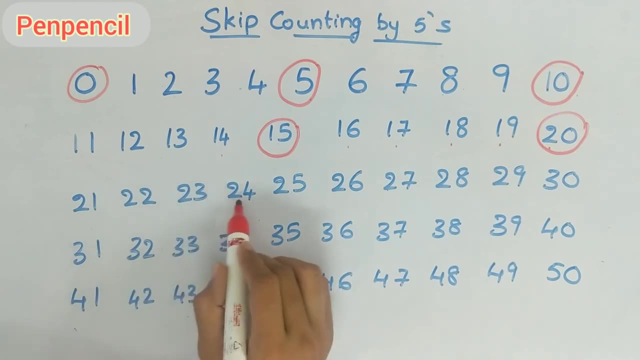 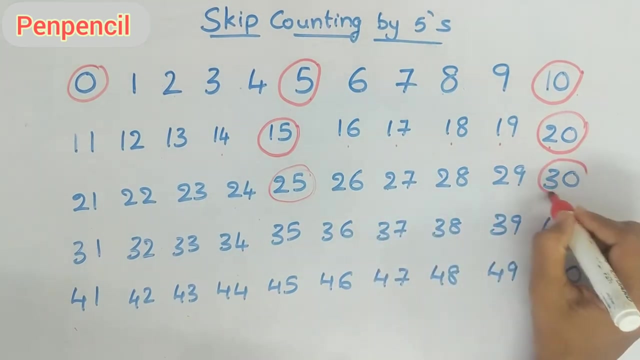 is 16,, 17,, 18,, 19,, 20.. That means 1,, 2,, 3,, 4,, 5. 20.. This way you have to circle. What is the next number? 1, 2,, 3,, 4,, 5. 25.. Next number is 30.. Again, 1, 2,, 3,, 4,, 5.. 35 is. 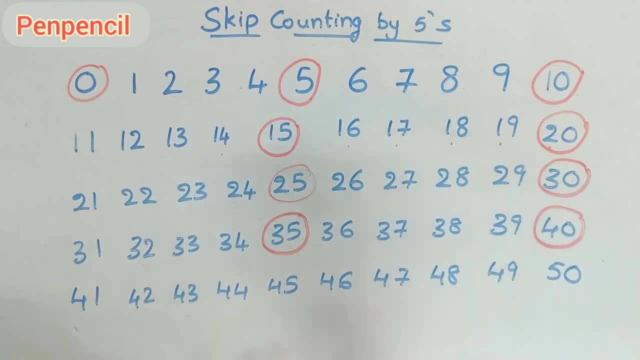 the next number, Again, 40.. Next two you have to do on your own. Ok, Now we will write once again what all we have circled. Ok, First number is 0,, 5,, 10,, 15,, 20,, 25,, 30,, 35,, 40,. 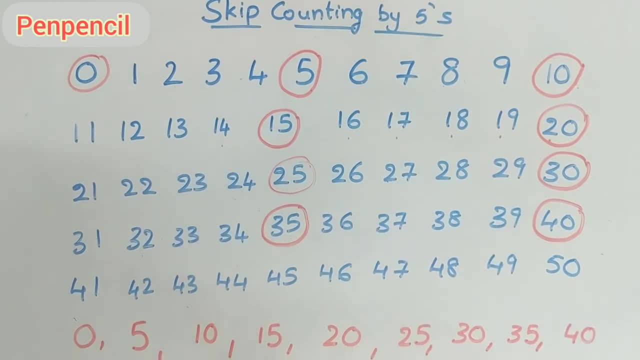 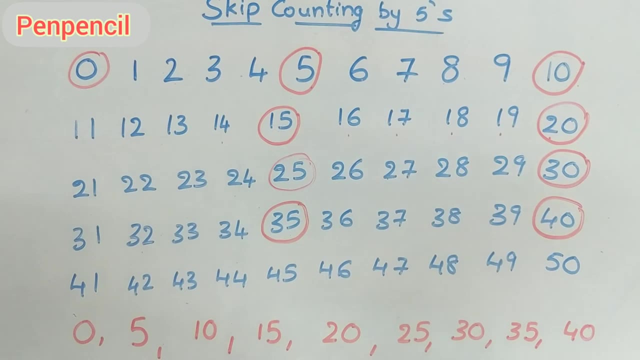 40, and 2 you have to fill. Ok, Have you understood, kids? Hope you have understood clearly. If you have not understood, please repeat it once again and learn again. Ok, kids, Thank you for watching this video. If you find this video helpful, please like, share and subscribe.